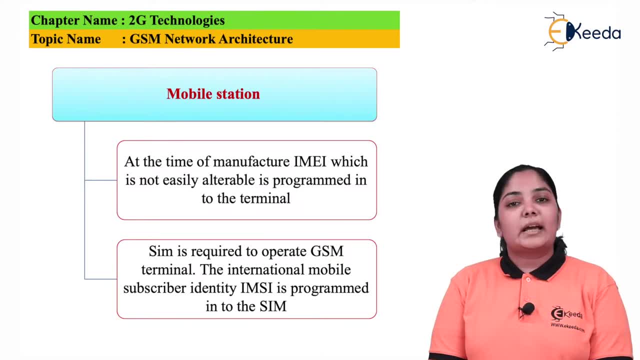 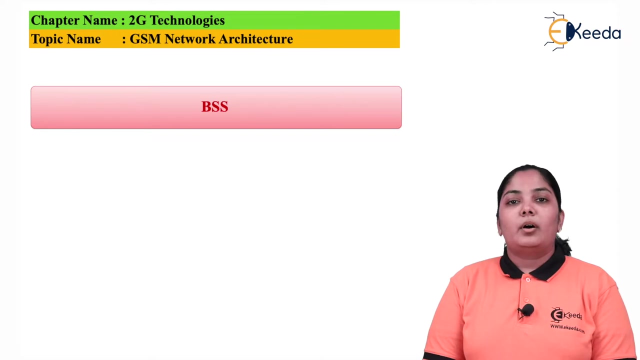 imsi number, which stands for international mobile subscriber identity number. this number is nothing but the actual mobile phone number that the user has. this number is incorporated into the sim card during the installation of sim card. the first part of the block diagram that is called as a bss base station subsystems. 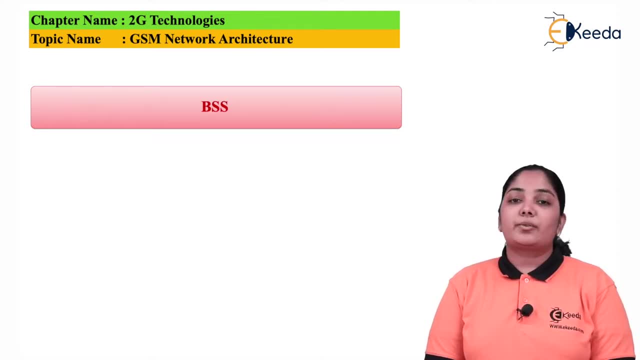 also has bts, which stands for base trans receiver stations, and it has bscs, which stands for base station controllers. as i said earlier, the bts are nothing but antennas that transmit and receive. they basically provide the radio interface for the communication to happen. there are multiple base 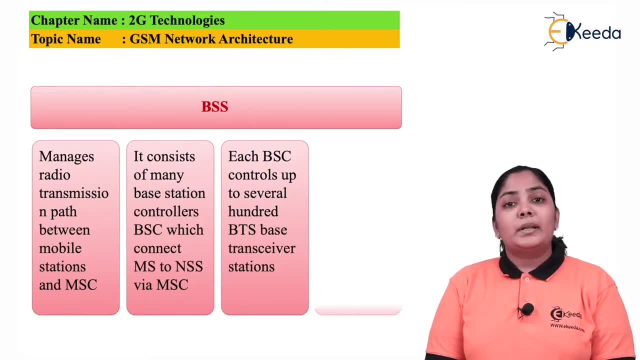 stations for individual base station controller. one base station controller can handle up to hundreds of trans receiver stations. the base station controller is used for communication between the msc and the mobile phones. the msc then further gets connected to other networks like pstn and isdn handoffs, if they occur between two base trans receiver stations within the same base station. 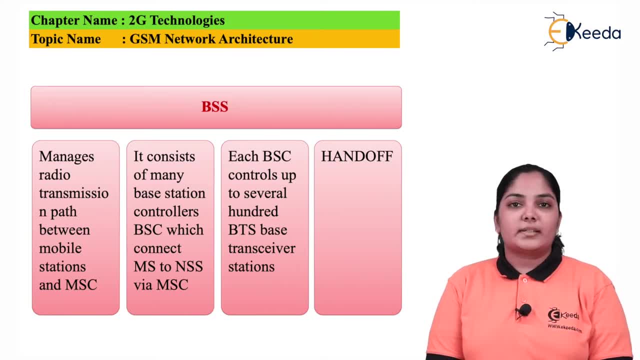 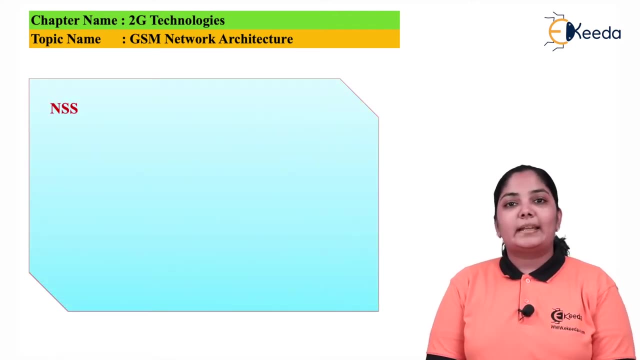 controller, then it is controlled by the base station controller itself or the bsc itself. if the handoff is between two base stations that are under different msc, then msc will take care of the handoff to occur. coming to the second part of the block diagram, which stands for nss, which is called as: 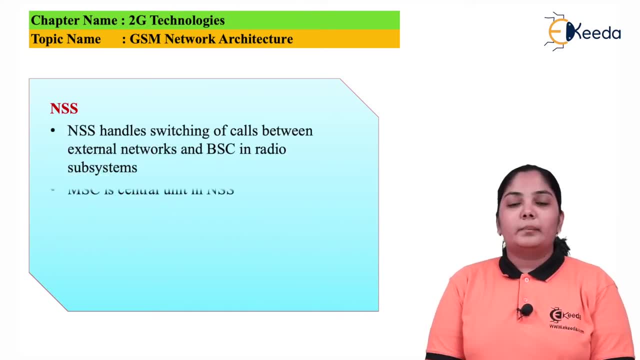 network switching subsystems. this part of the diagram basically helps connect the mobile phone to the other networks like pstn and isdn, and another one is called as msc, which stands for pstn and isdn, to the other networks like pstn and isdn. 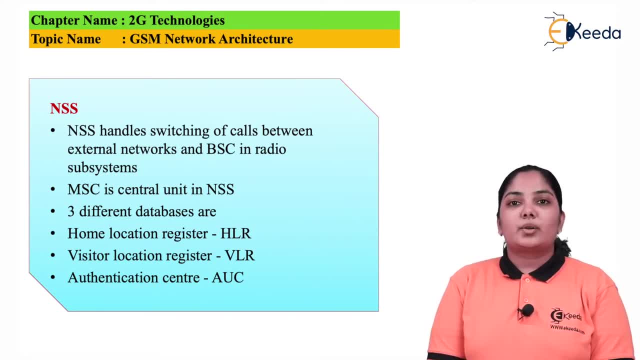 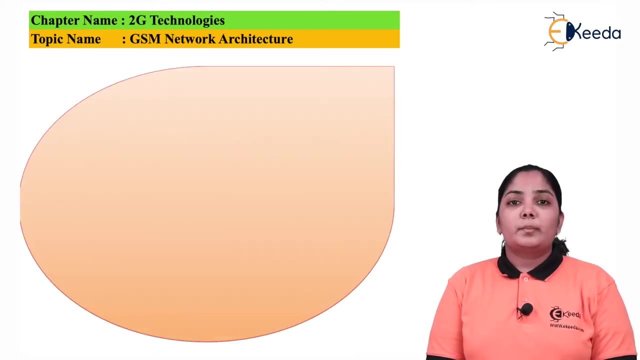 other data networks. this part consists of various registers called as hlr- home location register, vlr, visitor location register, auc, authentication center, msc and omc. let's talk about the hlr. hlr stands for home location register. this home location register contains the user's basic. 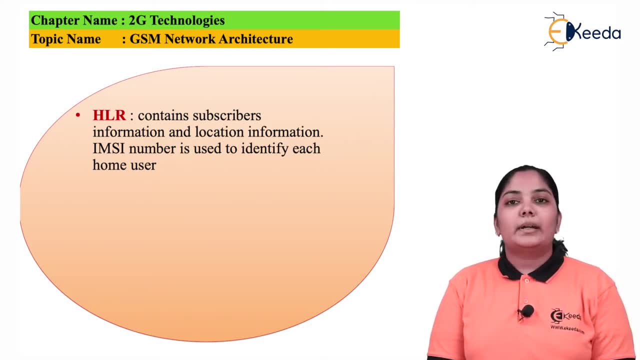 information like imsi number, which is called as international mobile subscriber identity, or the mobile phone number of the user. all the users that are in the home location get registered in this register, which is called as hlr. if the user is traveling from one place to another, then the 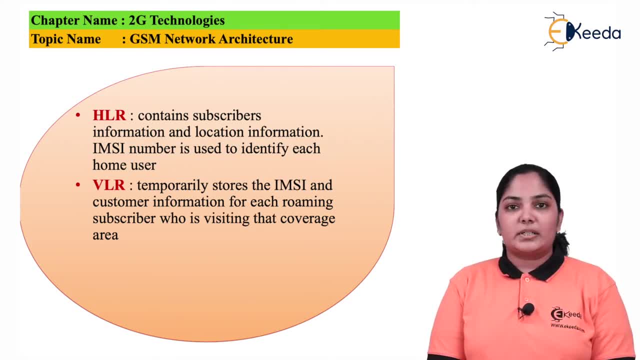 user gets registered into the visitor location register, which is called as vlr, the vlr will temporarily store a register in the home location register, vlr register. vlr register will temporarily store the IMSI number of the user because the user is just visiting that area and it will not be. 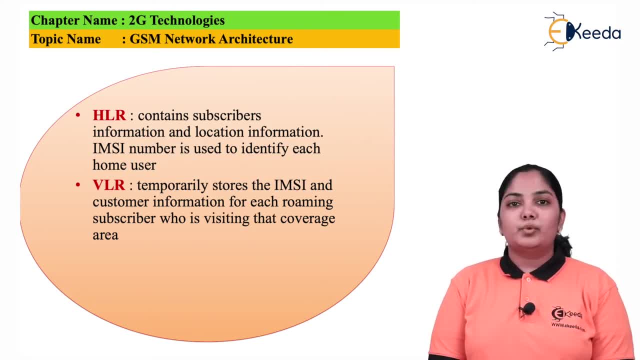 permanently stored, It might happen that the user again moves from that area to some other area. Hence the VLR temporarily stored the IMSI number and when the user will move from that location to some other location it will delete the IMSI number. The reason for the visitor location: 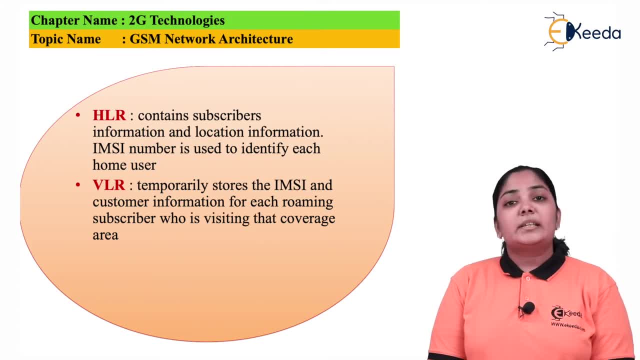 register to include the IMSI number is for the proper call routing when the user is at some other location other than its home location. The reason for the VLR to register the IMSI number is that the user should get proper calls when he is roaming out of its own home location area. If not, so then 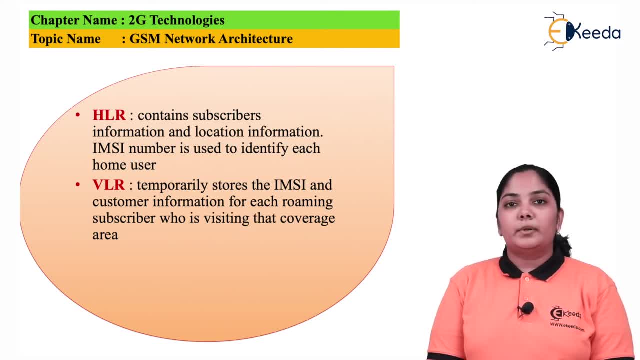 the user will not get the call request or will not be able to initiate a call when he or she is outside the home location. The VLR is also linked to multiple MSEs, called as mobile switching centers, so that the call may be routed from any location to the location at which the user is, The network switching subsystem. 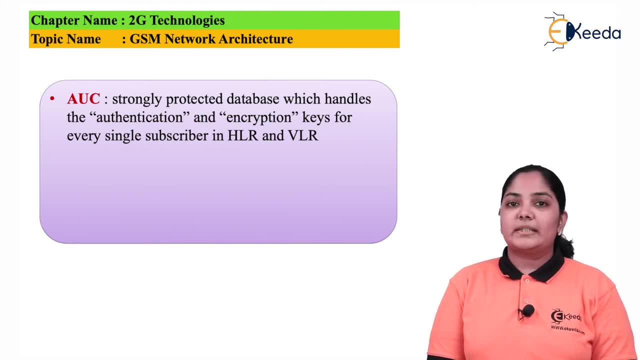 also holds a register called as authentication center. This authentication center is used to identify the stolen and the fraudulent phones. The authentication center also holds the authentication keys to the IMSI number. The authentication center also holds the authentication keys to the IMSI number and encryption information for every mobile phone user. Authentication center has a.